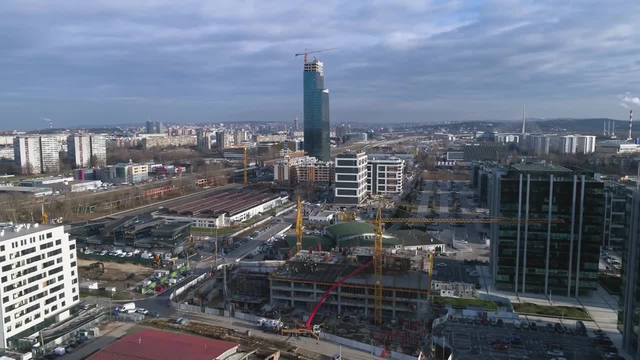 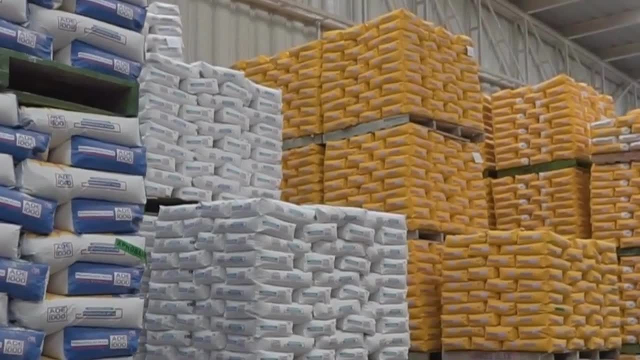 That's why it is impossible to calculate the exact cost of a project and that's why we tend to estimate in-state. and this is where the word estimation is coming from. Take an example: any building materials We can supply at different rates from different suppliers. And some specific materials, especially metals, are subject to monthly international price change. Usually we can negotiate the prices of the materials and all I know that. but this is done when you are procuring the material, not when you are estimating the cost of the 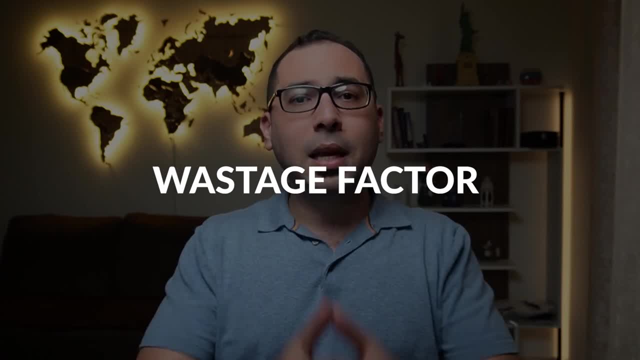 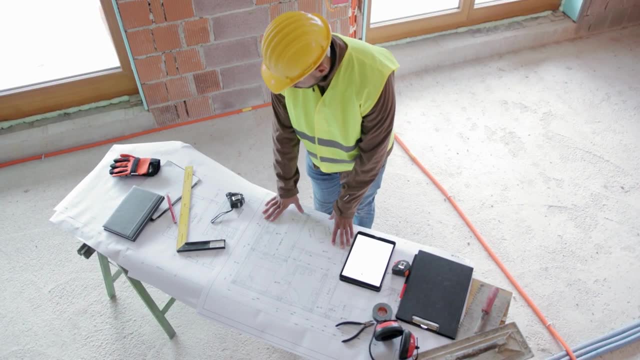 project in the beginning. There is also a wastage factor for all the materials in the projects and wastage is usually calculated from the shop drawings. But at the time of estimating the cost you might not have all the shop drawings ready yet, because the contract is not yet signed and usually shop drawings are prepared after. 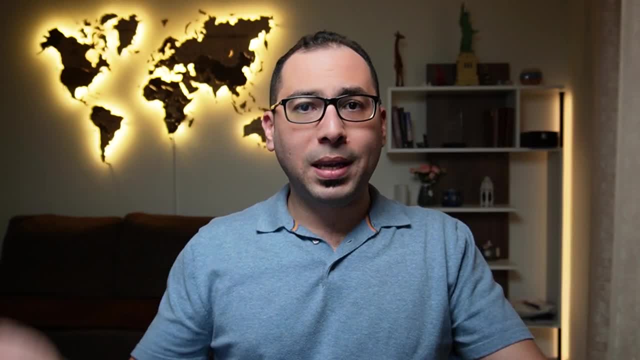 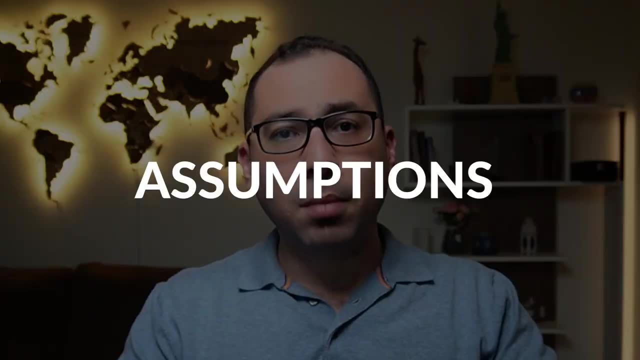 signing the contract. Even if the shop drawings are ready and wastage can be calculated, There is no guarantee that no materials will break during shifting or installation. So you have to start making some assumptions to account for that. Such assumptions is what we call the basis of estimate. 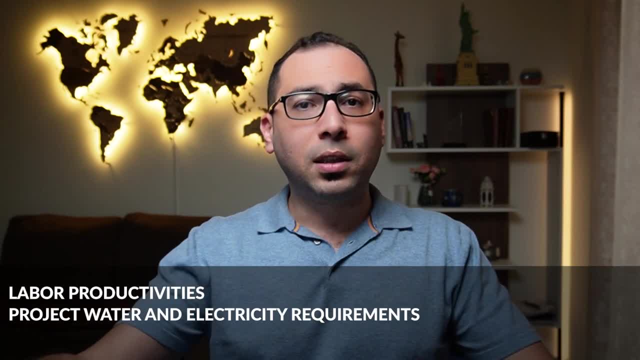 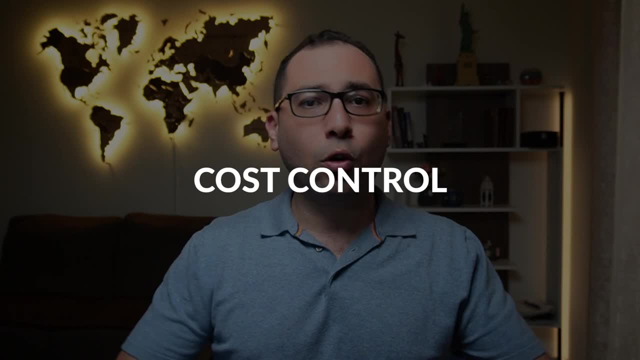 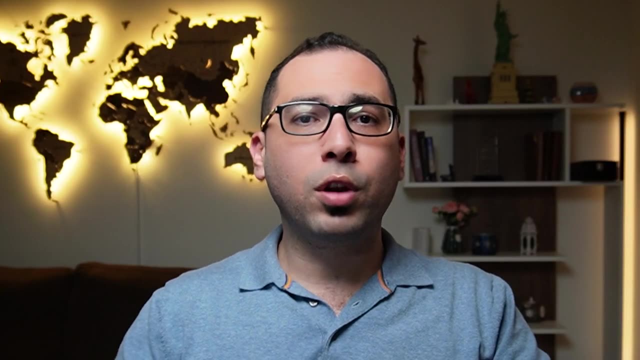 There are assumptions for labor productivities, project water and electricity requirements and the project staff requirements as well. Knowledge areas such as project management, planning, cost control. procurement contracts are there to control the project and its costs, but this is during execution, not during tendering. 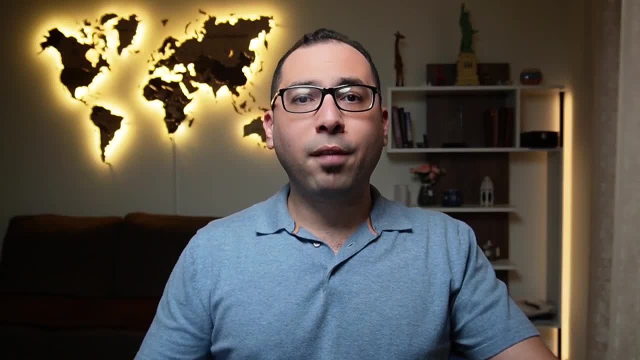 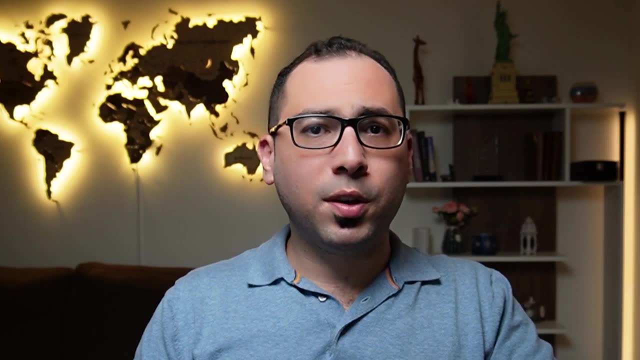 or estimating the cost, The cost of the project in the beginning. That's why we have to assume things and estimate the cost accordingly and that's why it is called cost estimation. And if we are meeting for the first time- I am Ahmed Adel and you are watching cost. 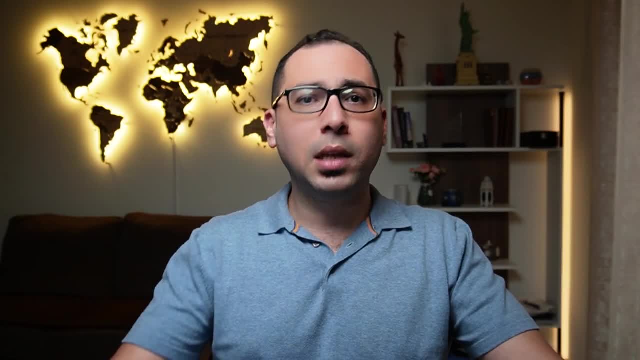 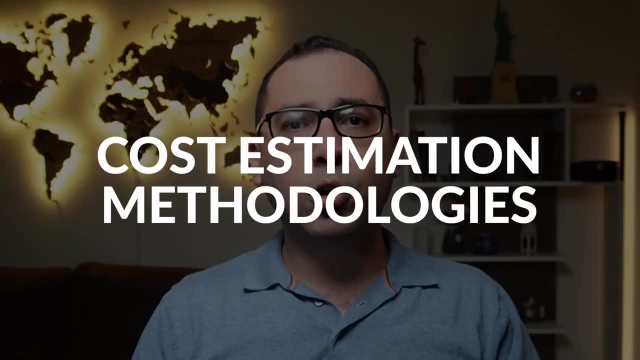 engineering professional, and here I help you develop the required skills and enhance your knowledge to elevate your cost engineering career. So if this is what you want, you can quickly subscribe Now. regarding project cost estimation methodologies, there are two methodologies used to estimate the cost of a project. 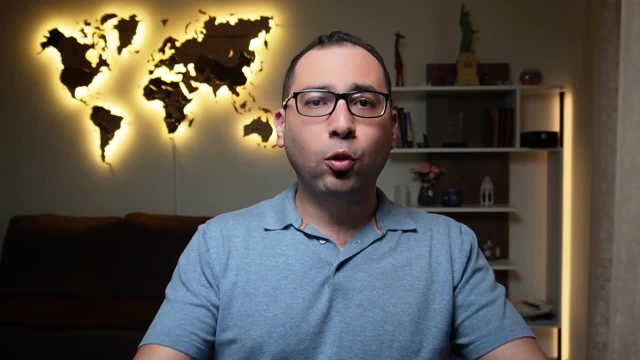 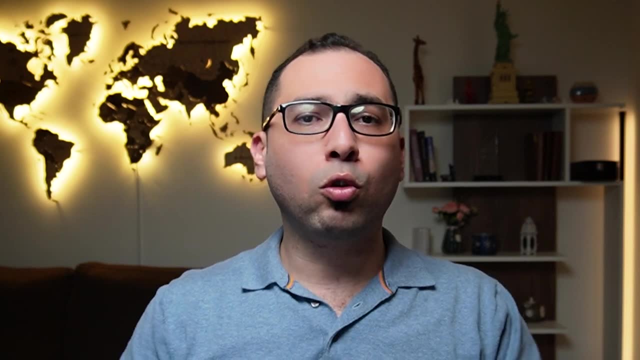 Conceptual and deterministic cost estimating And I have talked about them in details here on the channel in one of the videos. I'll leave the link to that video in the description down below in case you want to know the details and the differences between each of them. 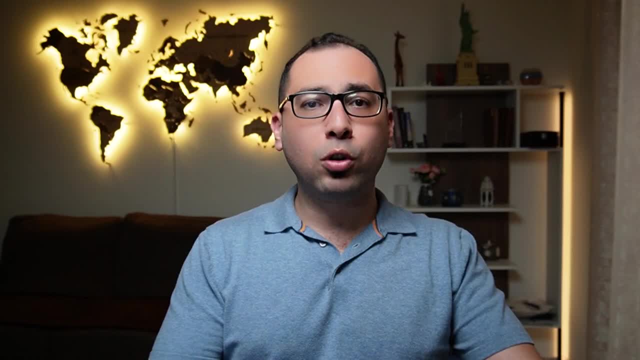 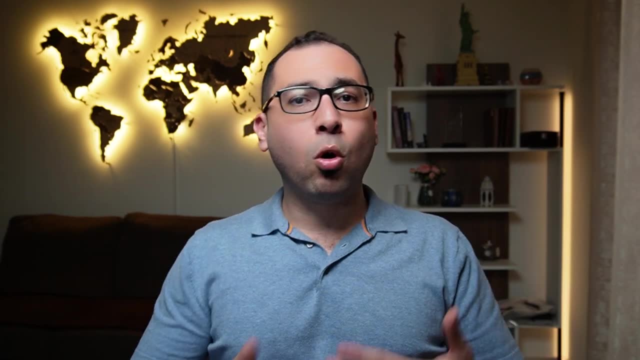 But, generally speaking, conceptual cost estimation is a methodology used to estimate the cost of the project when the scope of work is not very well defined, And it doesn't require much time or efforts to prepare, as it depends mostly on historical data and past experience. 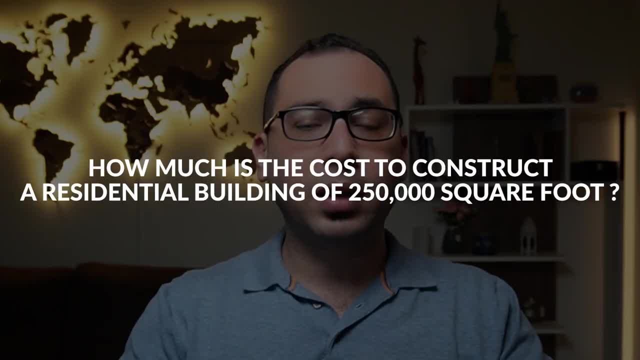 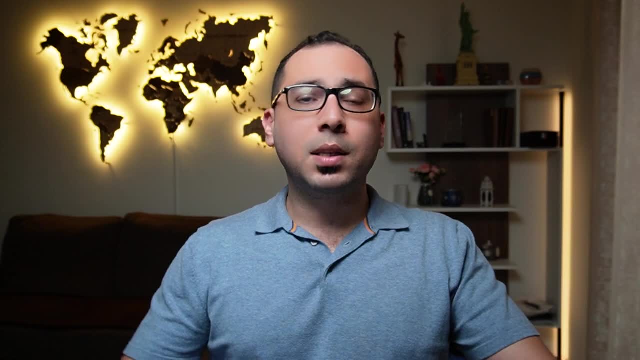 An example for that can be: How much does a project cost? How much is the cost to construct a residential building of 250,000 sq ft built up area? Well, if we know from our past experience that residential buildings cost around 250 dirhams, 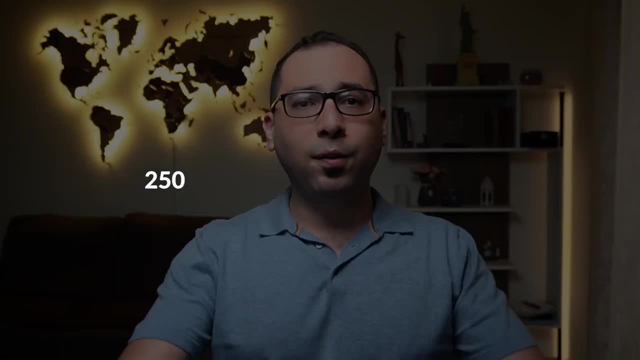 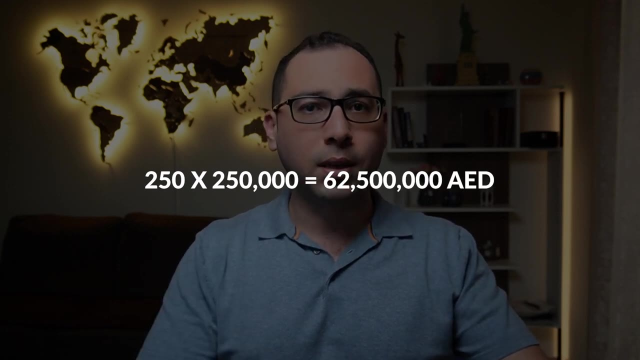 per square foot, then this building will cost around 250 multiplied by 250,000, which is equal to 62,500,000 dirhams, for example. In a very short time and using only the building built up area and the construction cost rate. 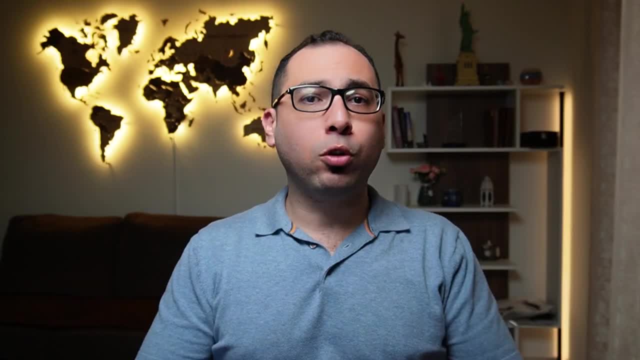 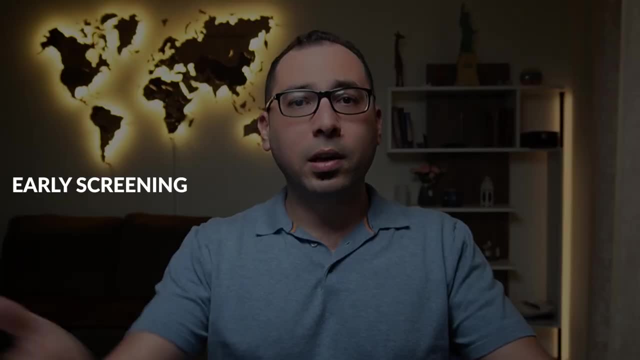 we can estimate the cost of the project. However, this is not an accurate estimate because we don't know anything about the project other than the built up area, which makes this type of cost estimation suitable only for early screening or budgeting purposes. On the other hand, deterministic cost estimation methodology is used when the scope of work 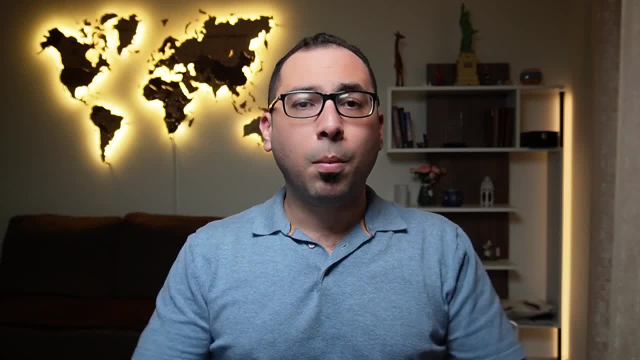 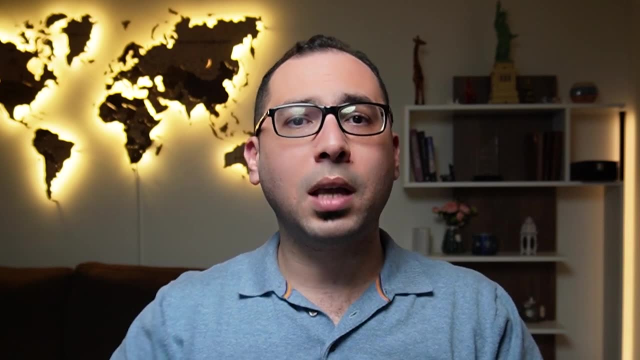 is very well defined and the project requirements are very clear, but it requires much time and effort to prepare it, as it depends on accurate measurements and market quotations and rate breakdown analysis for all the requirements. So let's get started. So, for the build up area, we need to prepare the required materials and services in the 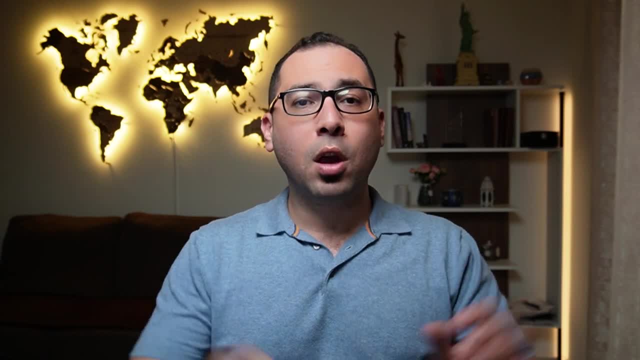 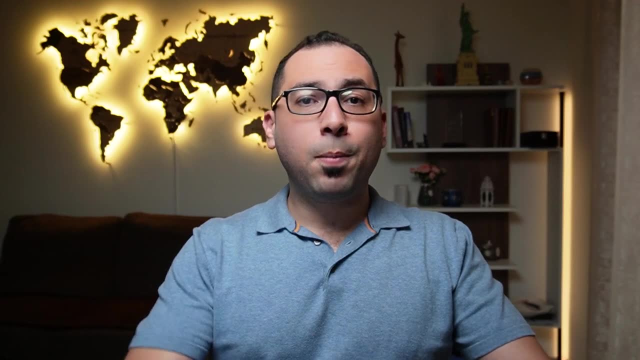 project, And to do all of this you need so much time and effort, but in the end it produces a very accurate estimate that you can use for bid submission and tendering. So when preparing a deterministic cost estimate, we need to be looking into the prices of the. 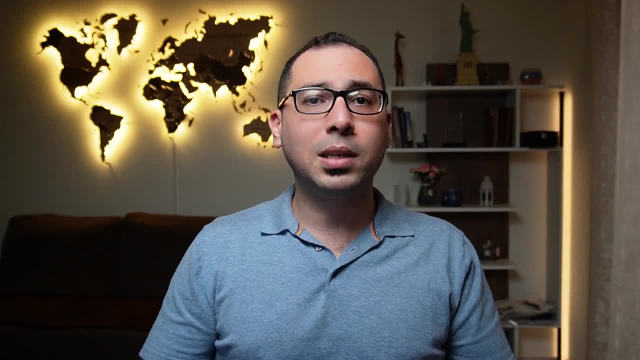 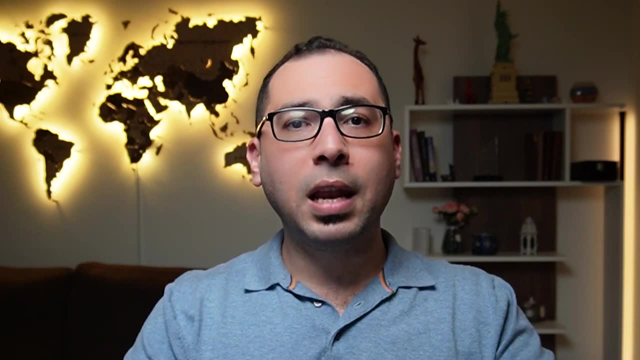 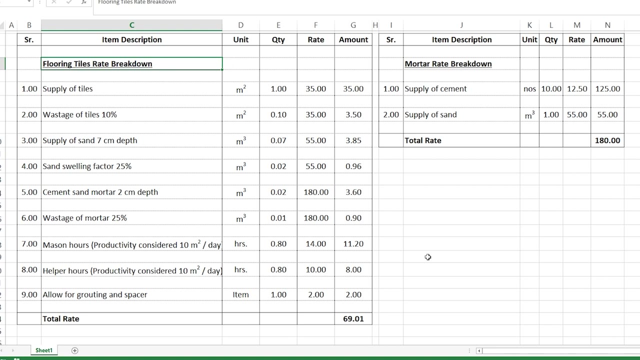 materials, equipment, manpower and subcontractors or specialists required for the project and, of course, the project general requirements as well. And now let us have a look on how the rate breakdown analysis looks like. As you can see here on the screen, we need the flooring tiles rate breakdown analysis. so, for example, first of all we need to supply the 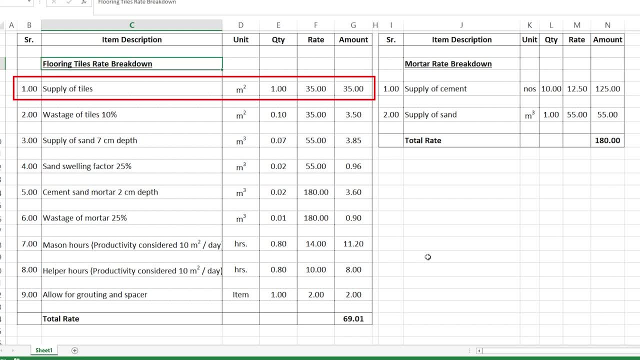 tiles, and now i am calculating the rate of one square meter of tile. so one square meter here multiplied by the supply rate of the tiles, which is 35, so 1 into 35, that's 35. then we need 10 wastage, and this is an assumption. so the quantity here will be 0.1 square meter multiplied by the. 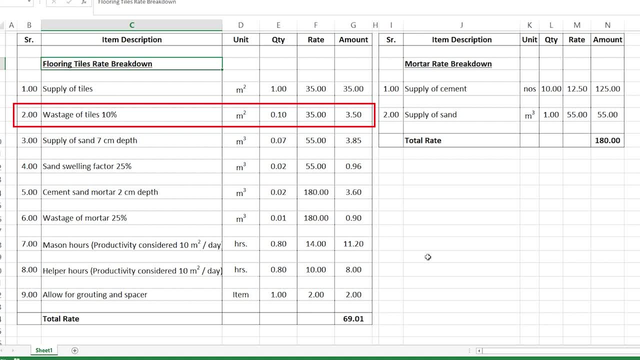 same tile supply rate, which is 35, and this will be equal to 3.5. then we need also supply of 7 centimeters sand. so 0.07 cubic meter multiplied by 55 dirhams, that's 3.85 for the supply of the sand. 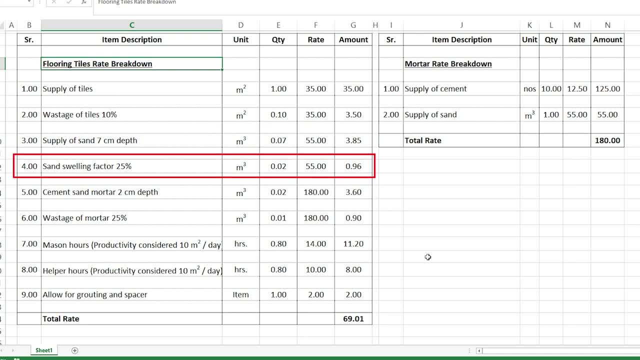 and also we have a swelling factor here of 25, so i'll just take 25 percent of the 0.07 and this will be 0.02, again multiplied by the same rate, which is sand supply rate 55. i'll emo ghe some 5.. theoritaly use 0.05 in the picture 825. so i'll take little 65, which will give you. 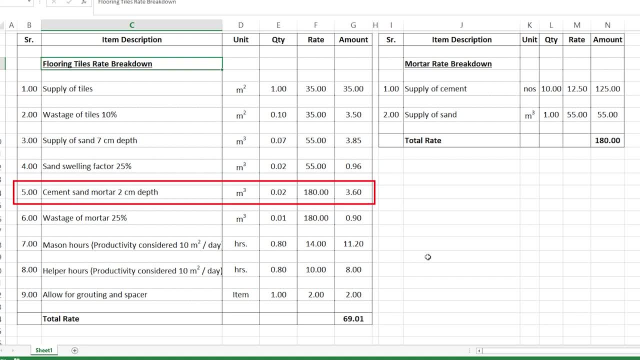 and that's 0.96. and also we need cement sand mortar two centimeters depth. so this is measured in cubic meter and the quantity will be 0.02 and this will be multiplied by the cubic meter rate of cement sand mortar. this rate we can calculate it here. as you can see: mortar rate breakdown. 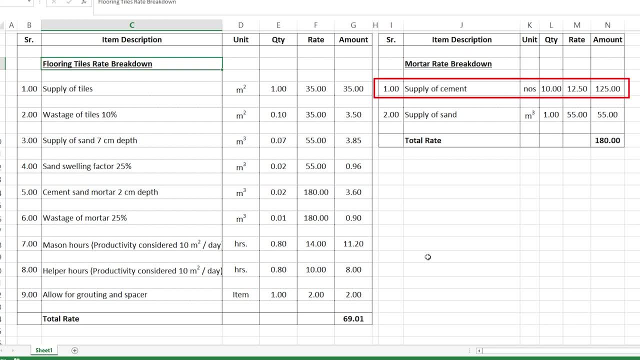 to produce one cubic meter of mortar we need cement tin bags and we need sand. one cubic meter. so 10 bags of cement multiplied by 12.5, that's 125. and for the sand we need one cubic meter into 55, so that's 55. so 125 plus 55, that's 180 here. so i'm just putting this rate here multiplied by. 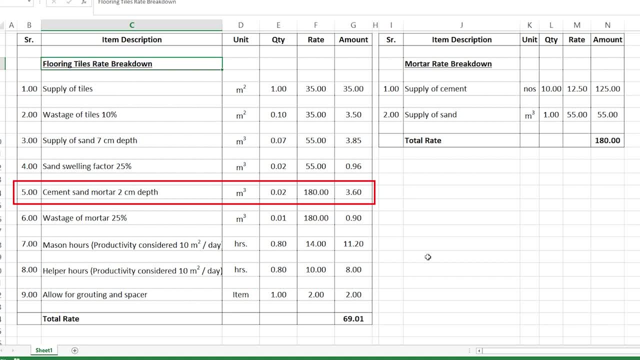 the 0.02 cubic meter, which is the quantity of mortar required. that's 3.6, and we need 25 wastage of mortar as well. so 25 percent of the 0.02. here i have 0.02 one- it's just because of the approximation, of course- and the rate is similar: 180, so 0.01 into. 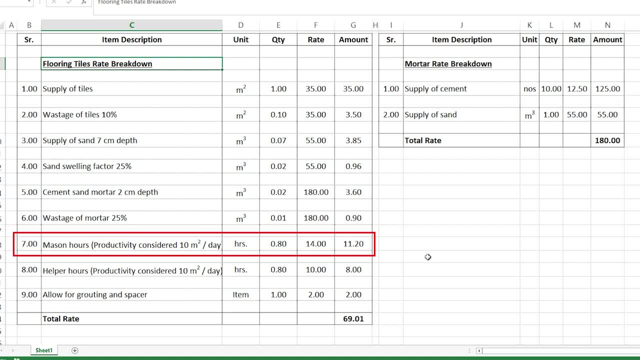 180, that's 0.9, and you need mason hours here. an hour to install one square meter of tiles. you need 0.8 hour and this is the hourly rate, 14 dirhams. so we need 11.2 for the masons who will. 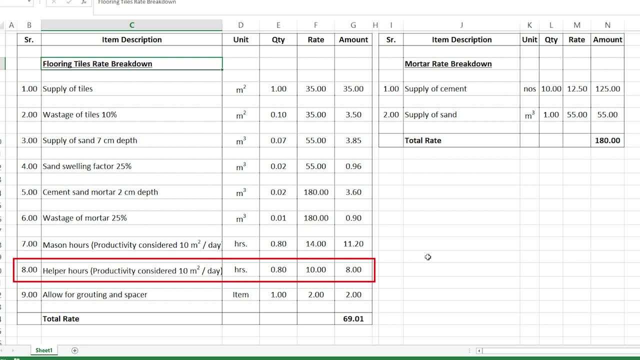 install and we need unskilled labor or a helper hour also to help this mason, and this will be again 0.8 of an hour multiplied by the hour, and this is the hourly rate multiplied by the hour, and this is the hourly rate of a labor, which is 10 dirhams. so that's 8 dirhams, and then we can allow. 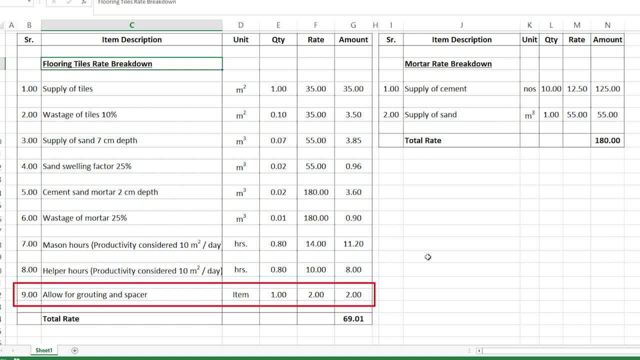 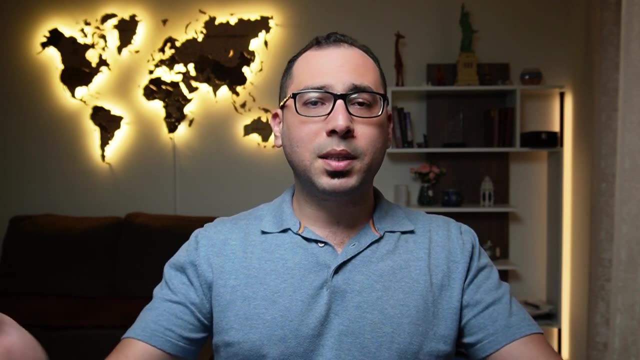 something for grouting and the spacer. so it is just an item and i am allowing two dirhams here for this. so the total here is two and the submission of all these is 69 or 70 dirhams. so this is how you calculate the rate of an item when you are going for a deterministic cost estimation.